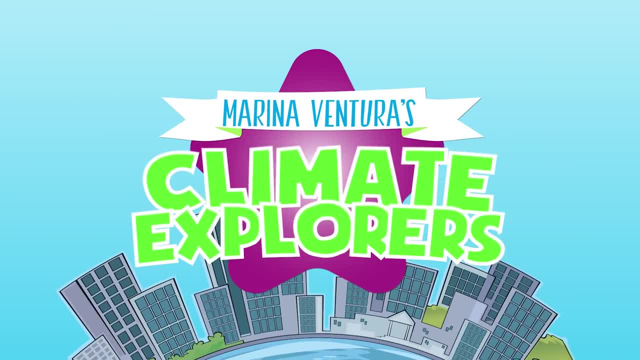 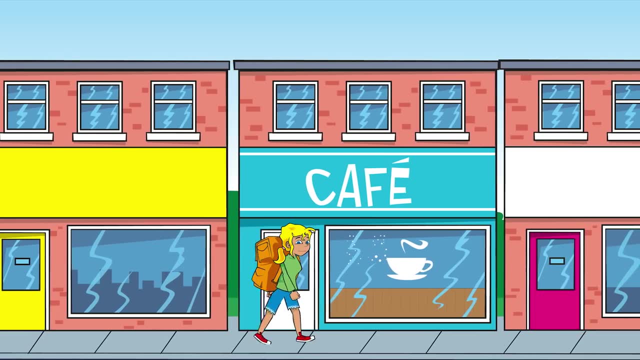 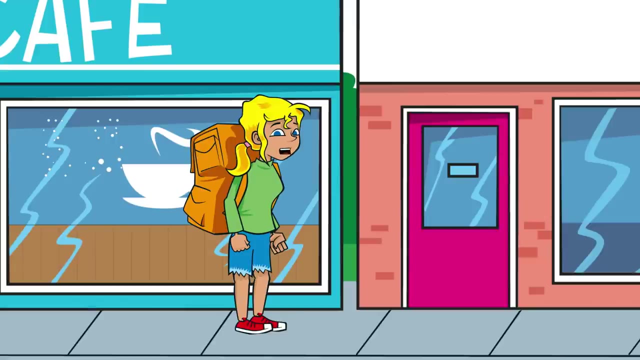 Hi there, Marina Ventura, here Now, as we've been finding out, when you hear the words weather and climate, you might think they mean the same thing, but they're quite different. Isn't that right Maffie? Hi Marina, Yes, that's correct. It might be rainy today or it might be sunny, That's. 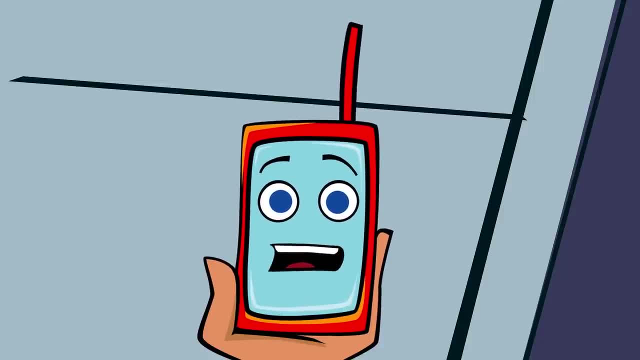 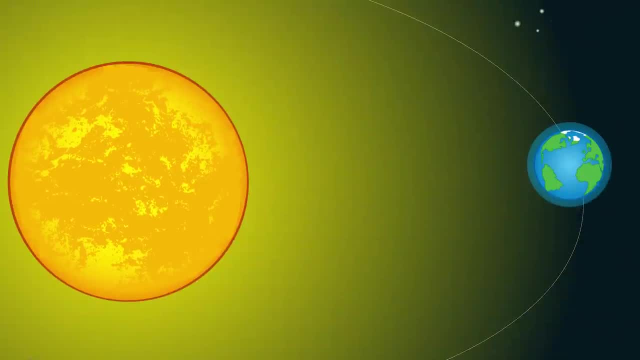 the weather. But climate is the pattern of weather in a place over a much longer time, And different parts of the world have very different patterns of weather. Why is that? The Earth's climate is driven by energy from the sun, which arrives in the form of heat. 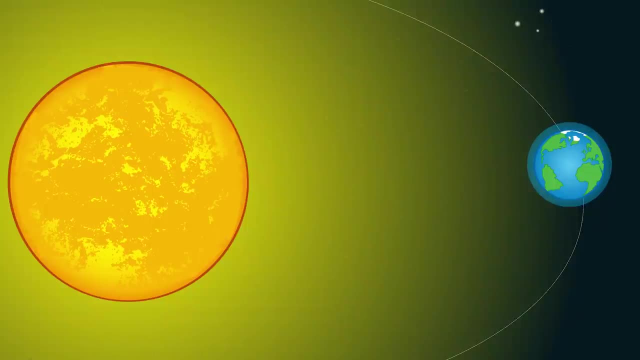 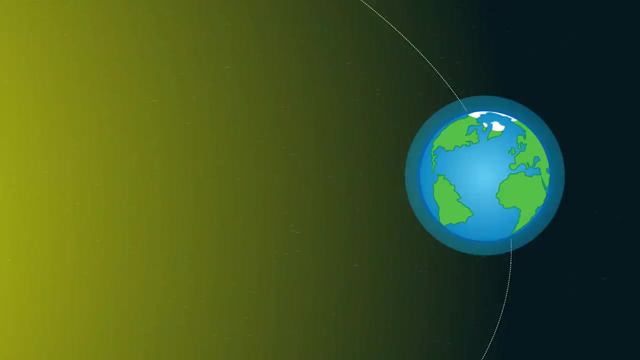 Half of this energy travels through our atmosphere and reaches the Earth's surface. The other half is either absorbed by the atmosphere or reflected back into space. Because the Earth is a sphere, the sun's rays reach the Earth's surface in polar regions at a much. 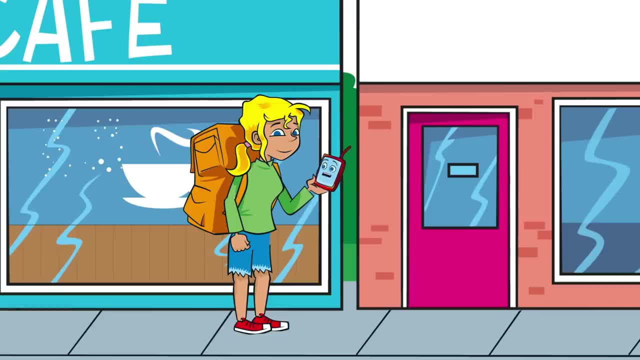 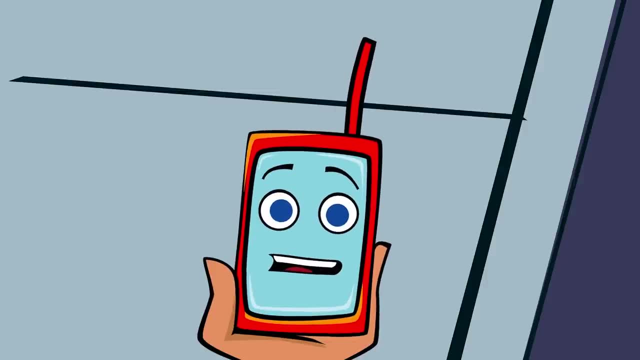 more slanted angle than at the equator. So, straight away, we know that the sun's rays reach the Earth's surface. We know that the poles are colder than the equator. Now, when things aren't in balance, nature likes to even things out. So the extra energy at the 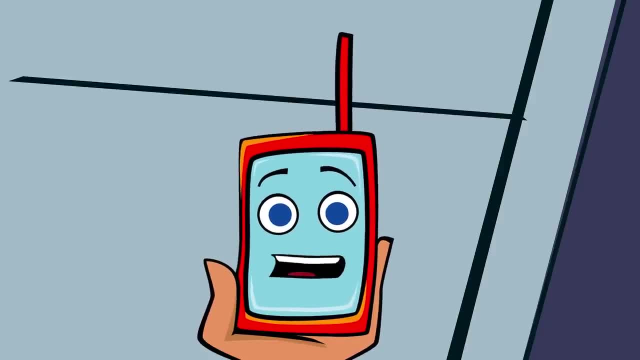 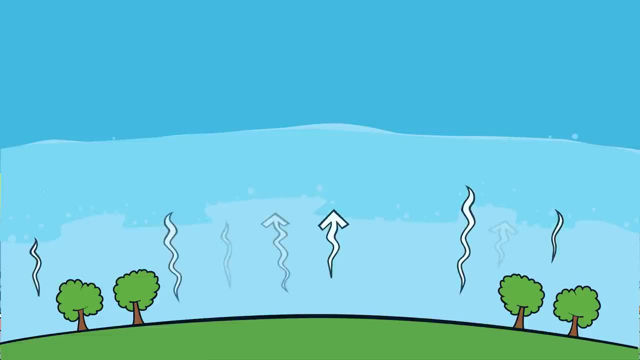 equator needs to be spread across the planet, And it's this that creates different climate zones across the world. Warm air rises at the equator and moves toward the poles, Where warm, wet air rises, we get thunderstorms and tropical rainforests, And where air sinks. 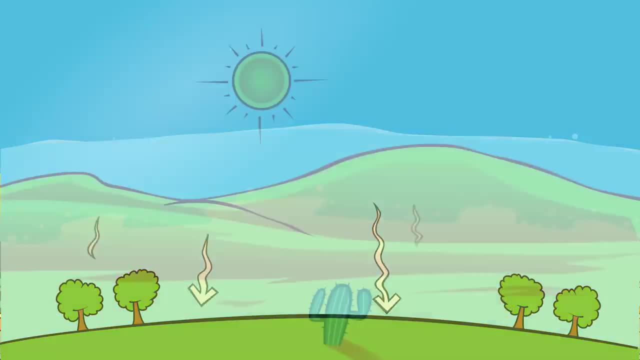 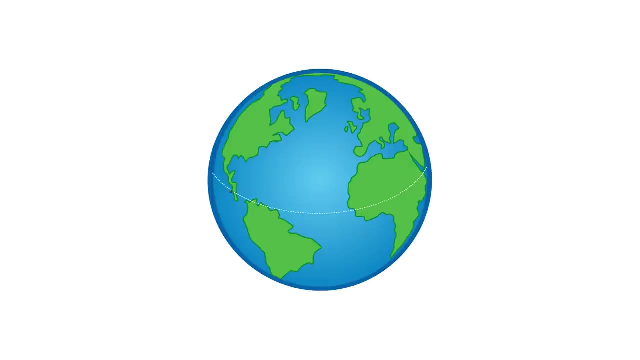 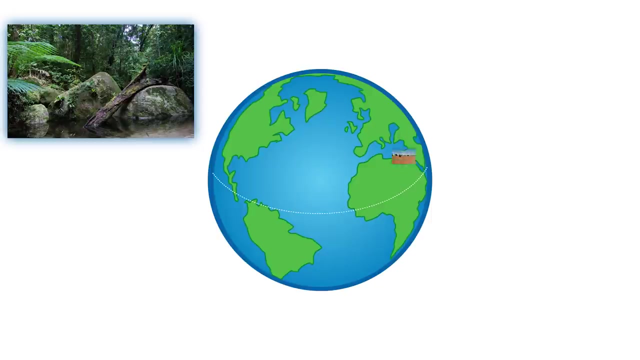 it stops clouds from forming, So it rains less, even making deserts. How many climate zones are there and how do they differ? Well, around the equator we have tropical climates which are hot and humid. This is where you'll find the world's rainforests. Then there are arid or dry climates, like 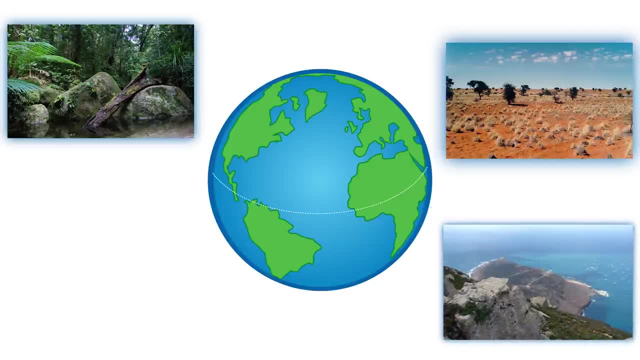 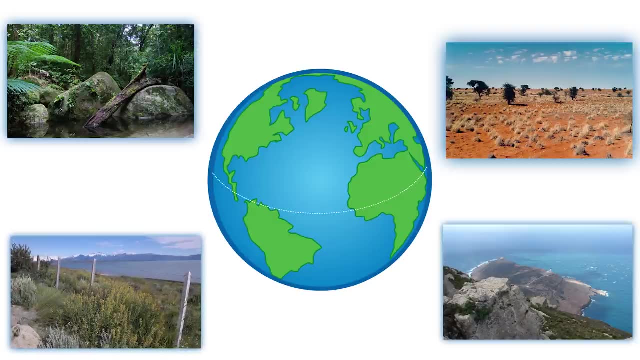 you'd find in deserts. Next is Mediterranean, with hot, dry summers and cooler, wetter winters, And then there are temperate climates. That's what we have in the UK, isn't it, Where summers are mild and winters aren't. 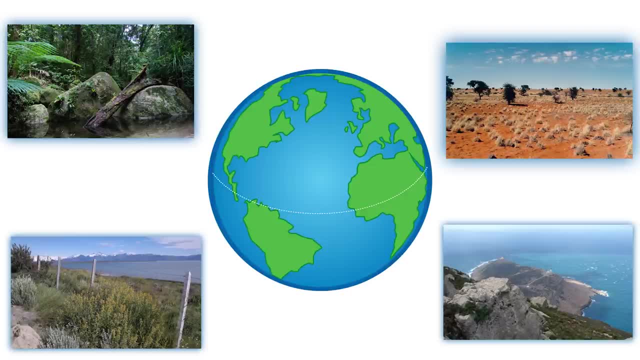 too cold. That's right. In areas that are a very long distance from the equator, there are arid climates, And if you're a long way from the sea, the climate is continental, with long cold winters and short hot summers. Finally, there's polar climates, which experience long periods. 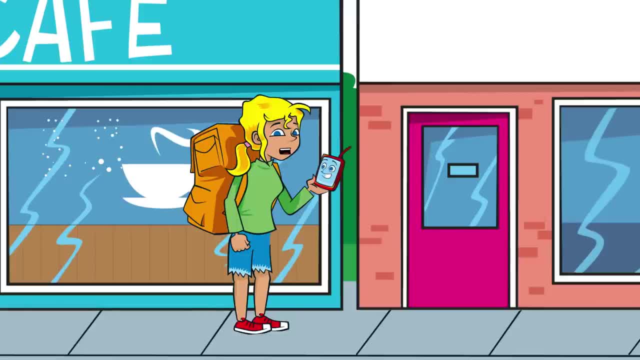 of extreme cold. Hang on though. I've been to countries like France and Italy in the Mediterranean and, depending upon where I am, I've experienced very different weather conditions. They have lots of snow in winter, and some of their mountains are even snow-covered all year round. But they also have beautiful weather conditions. They have lots of snow in winter and some of their mountains are even snow-covered all year round, But they also have beautiful beaches- great fun during the hot and dry summers. So if you've got both snow-covered mountains and hot beaches, does that mean they don't? have a Mediterranean climate? Of course not. It just means that local climates in a country can be different to the region's climate. This can be for lots of reasons. High places like mountains tend to be colder, because the air is cooler the higher you go. 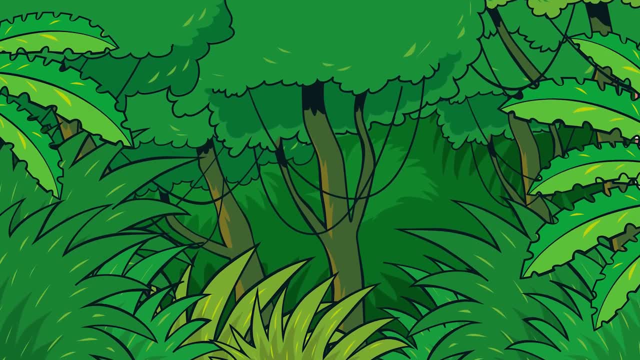 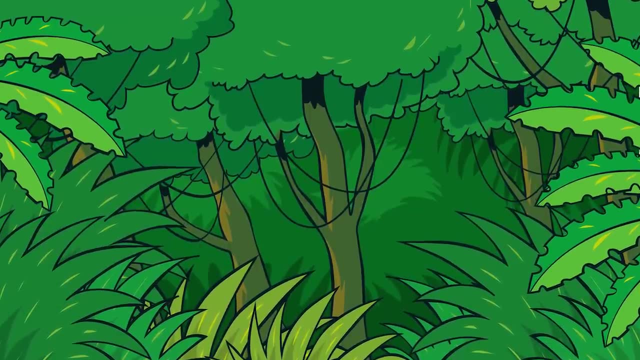 Vegetation can also affect the local climate we experience. In extreme cold, we experience more of a hot summer. In equatorial rainforests, dense vegetation blocking the wind, combined with high temperatures and rainfall, means it's a very humid place to be Where there's no vegetation, the air can be much drier and the wind can blow. In busy cities, the air temperature is often warmer than the surrounding countryside, particularly at night time. This is due to buildings and roads absorbing heat during the day and giving it off at night. 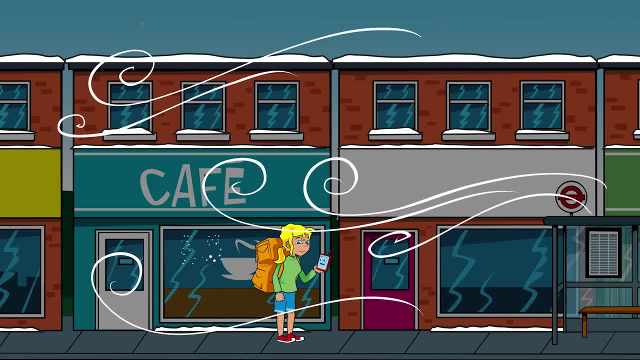 Another thing that can affect a local climate is the wind. It might be that part of the air is too hot. It might be that part of a country frequently catches wind from another region. This is called a prevailing wind. If it's coming from a hotter place, this might raise temperatures. 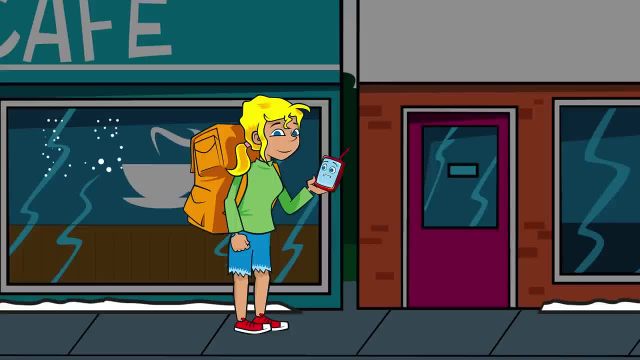 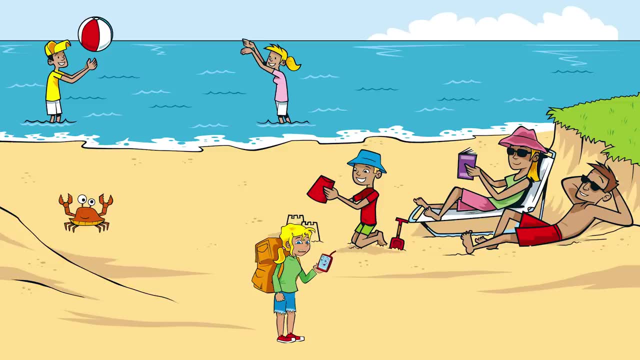 Or if it's from a colder area, it will cause the local temperature to drop. I think I want to be back on the beach. This wind's coming from a very cold place- Lovely Time for a dip. Even the oceans have a part to play in influencing our weather and climate. 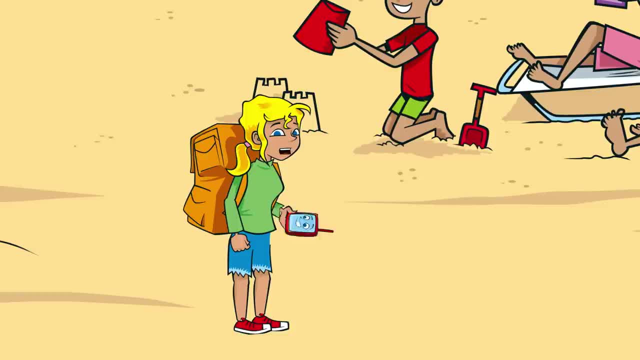 As we shall find out later. Thanks, Mappy. And just because a place has one climate doesn't mean it won't change Climate. scientists take measurements over long periods of time to track patterns in temperature and rainfall. These help us know what to expect today and in the future. 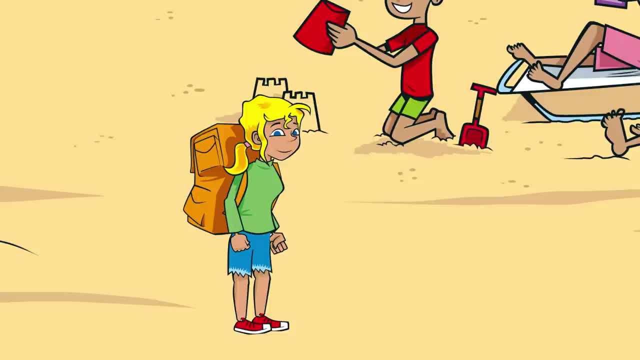 but are also a great way to see what changes have happened in the past. Amazing to think that 20,000 years ago the UK would have been in the Ice Age and our climate here would have been similar to the polar climates that we see today. 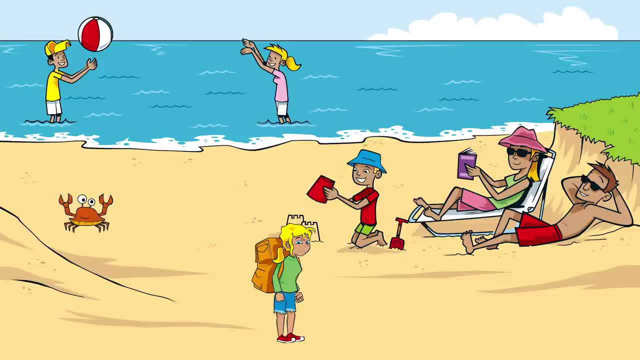 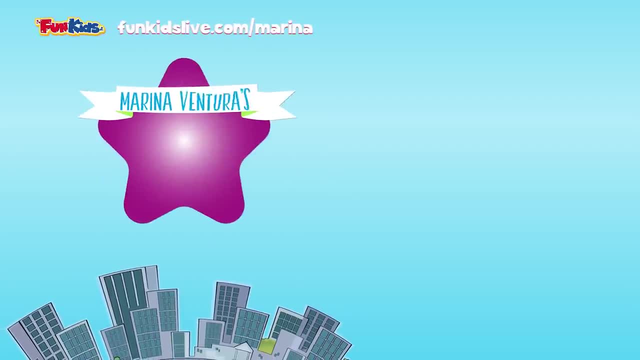 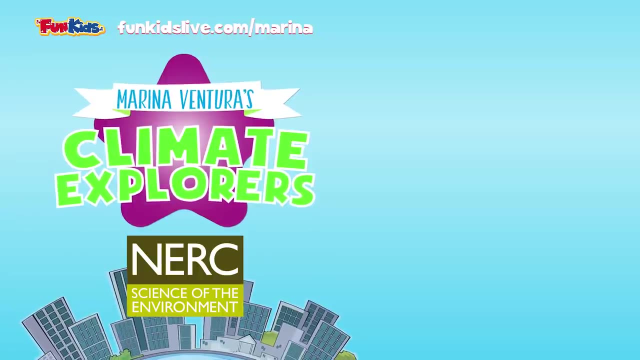 Cold enough to have a pet polar bear. Join us next time when we'll be finding out about how and why climates change: Marina Ventura's Climate Explorers, Supported by the Natural Environment Research Council, The science of the natural world. Find out more at funkidslivecom. slash marina.